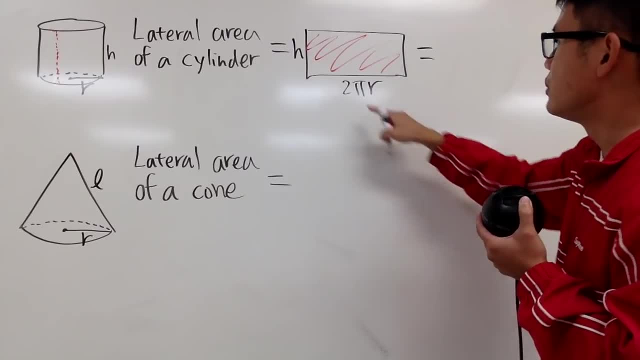 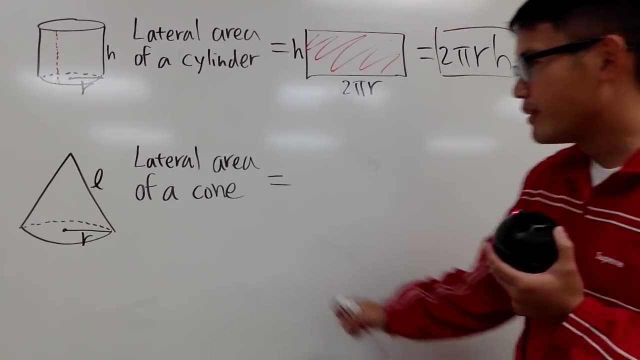 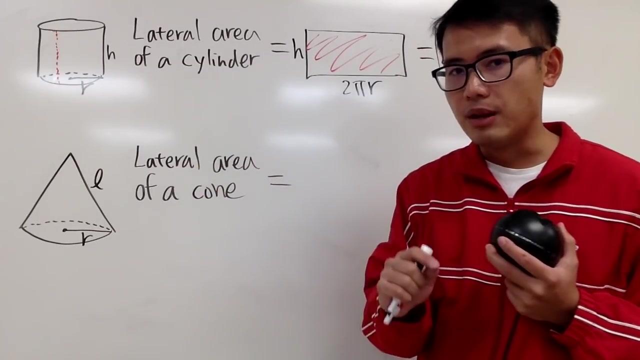 And now you have this rectangle. The area of this is just this times that, which is 2 pi r times h, And you are done. Now. this is slightly more complicated and we'll focus on this right here. For the lateral area of the cone, it's the following: 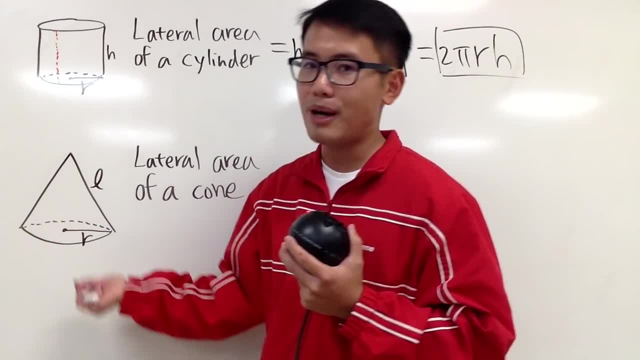 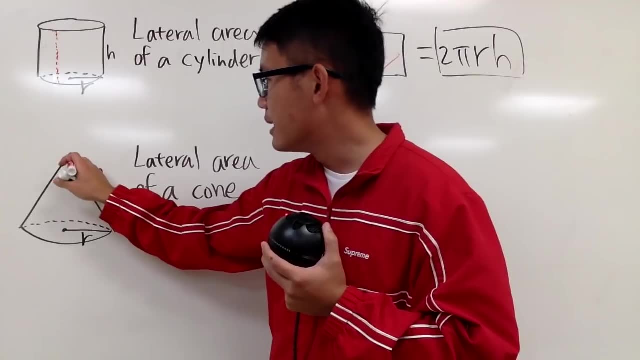 I want just around the side. I don't care about the bottom. The bottom is just the area of the circle, so that's easy. Let's just focus on the side. Well, well, I will first make a cut like this, but this time you have to cut it like standing right. 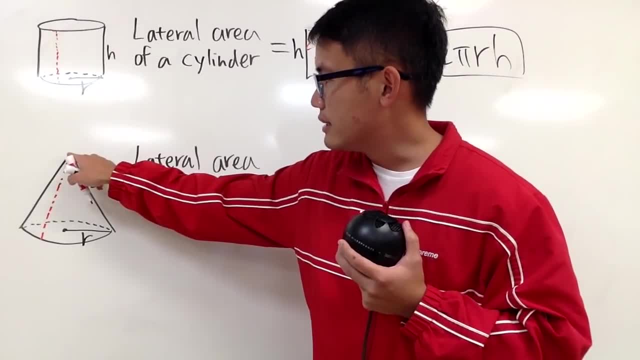 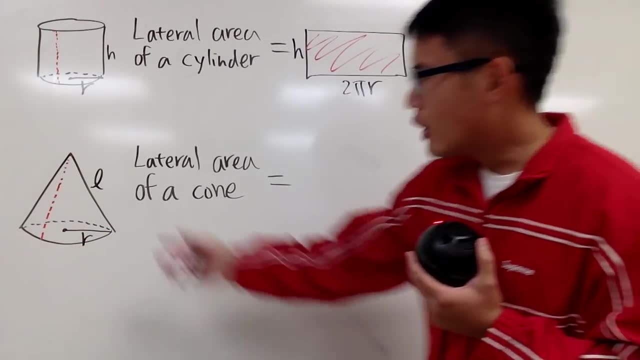 This is not straight anymore. The l is the slant distance And then the r- right here, it's the radius. It's the radius of the base circle. So I make the cut. I'm going to open it. The picture is going to look like this: 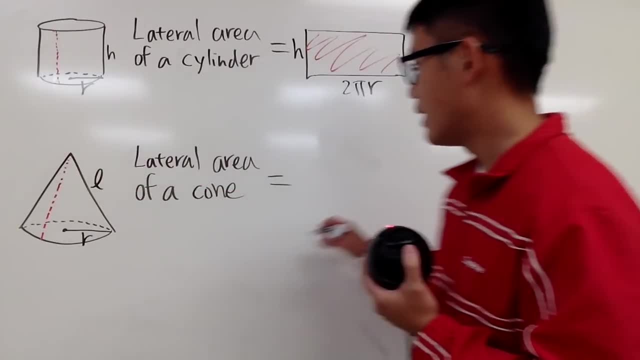 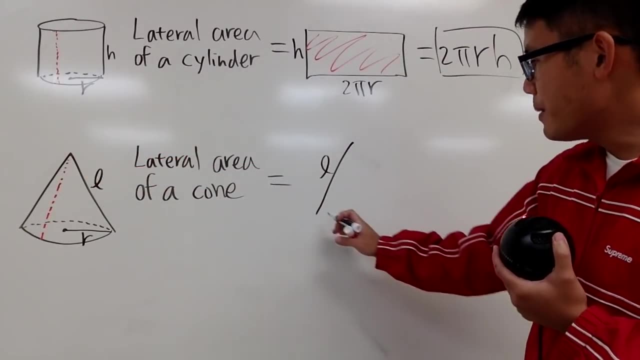 Now let's see, This is l, So I will also keep it like this, l like that. So this right here is l, This right here is l, And then, if I open it, in fact we'll get like a sector. 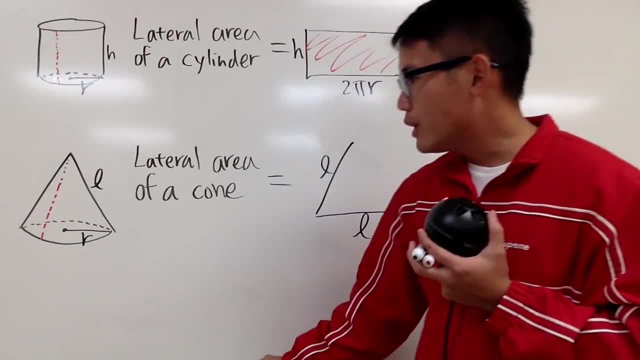 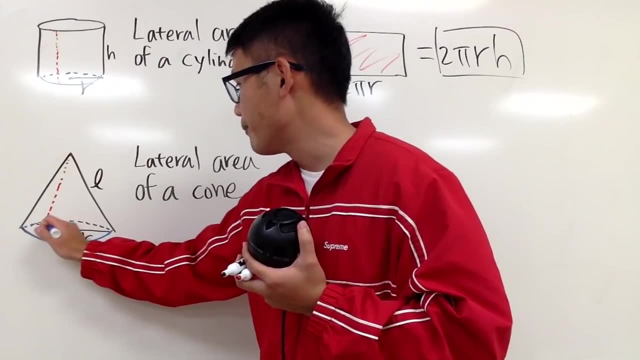 This is also going to be l And what you are going to get on the bottom part right here. as you see, this is the center, This is the bottom, with the base circle. You have to open it and that's going to be around the side right here. 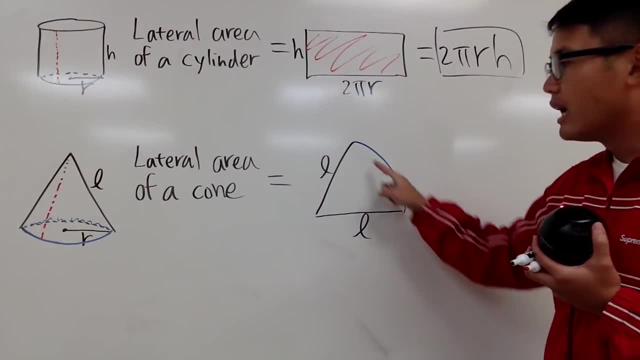 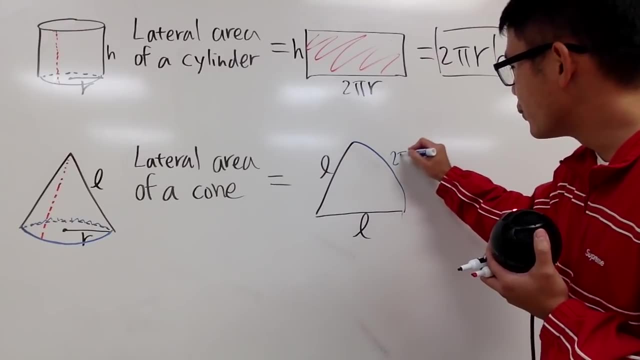 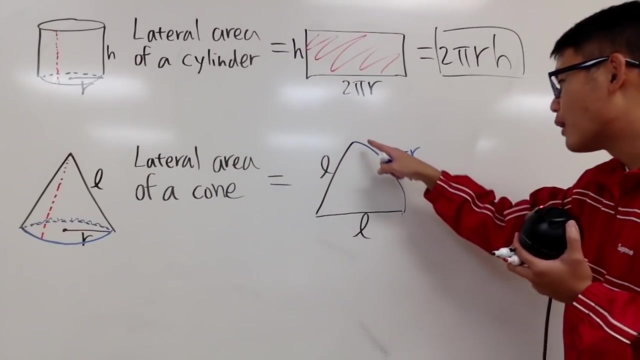 And in fact you will have an arc. This arc is precisely the circumference of the bottom circle. So this right here will be 2 pi r. This is the circumference of the circle on the base. Of course, that will be 2 pi r. 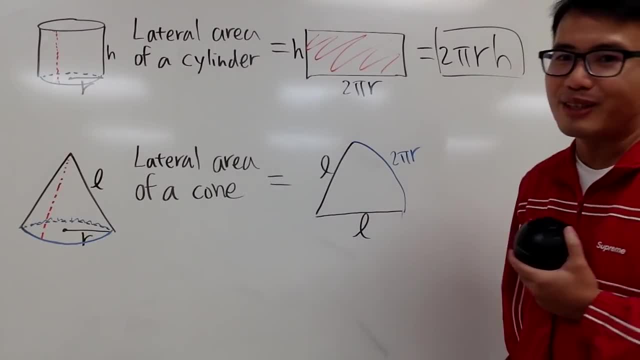 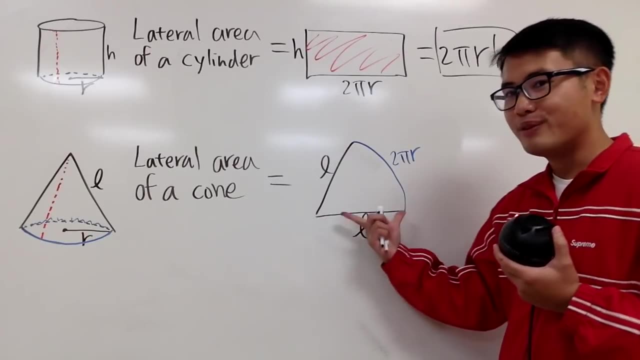 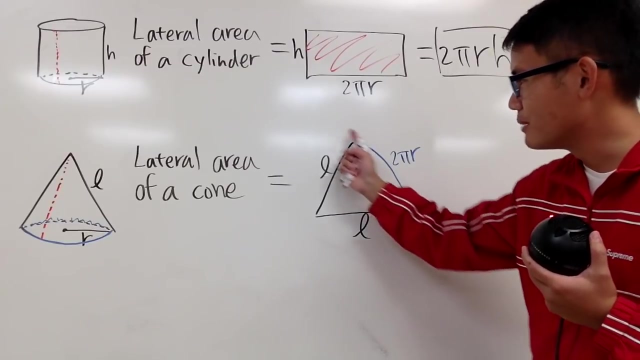 And now I would like to know how can we find the area of this sector? Of course, to find the area of the sector, we need two things: The radius of the sector. imagine if you have a whole circle. This time the radius is actually l, because you are talking about a whole circle. 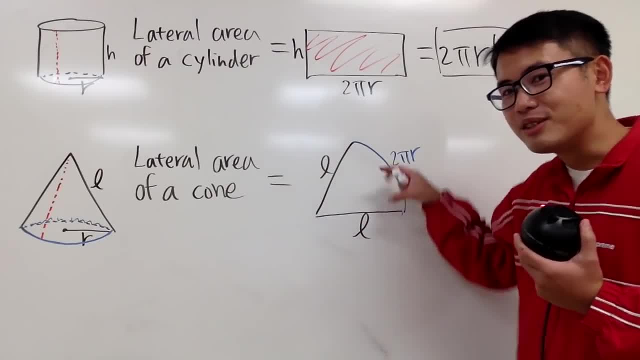 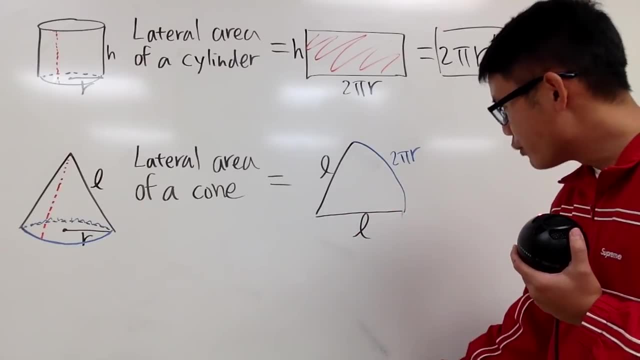 Just imagine that if I just have a whole circle, This is just a piece, just like a slice of a pizza, And I also need to know the angle right here. So let me put that down: I need to figure out the angle. theta right here. 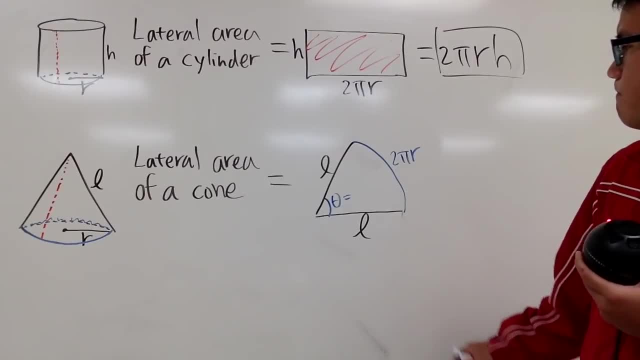 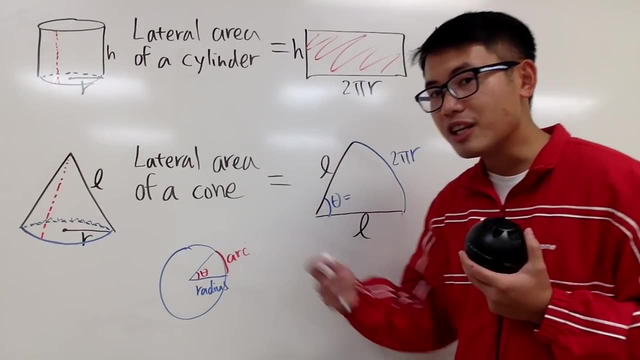 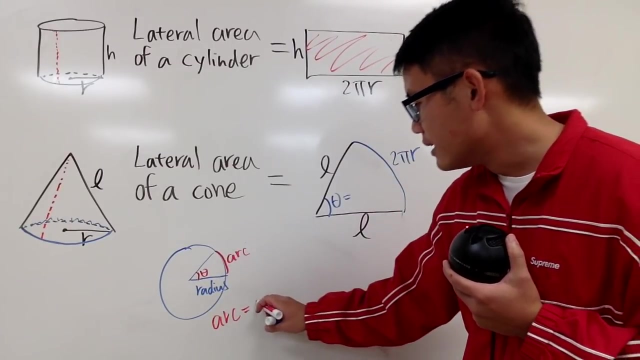 And now to figure out this angle, I have the arc, I have the radius. Let me remind you, guys- And you can check out my other video- I showed you that the length of this arc is equal to just the radius times the angle theta. 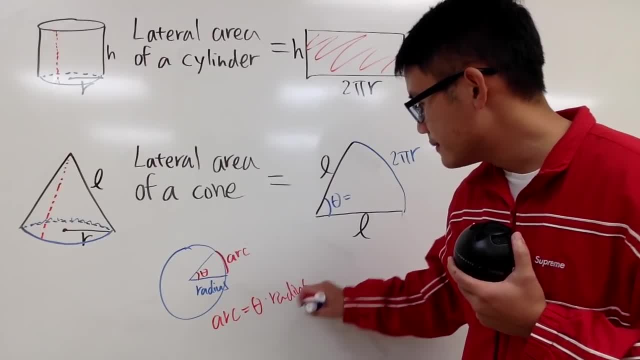 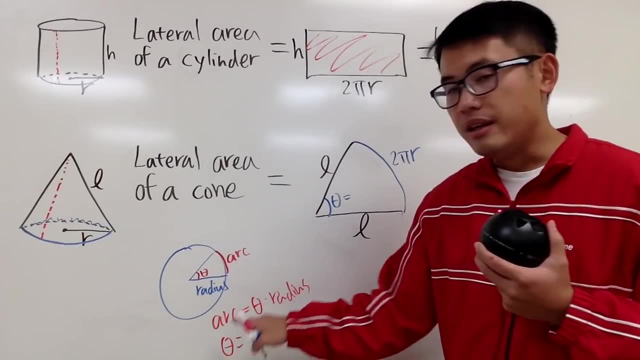 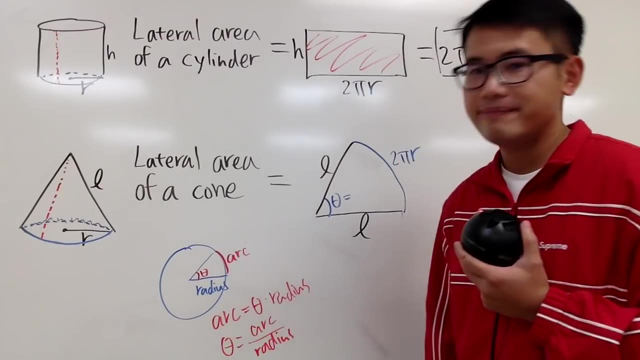 So I will put down theta times the radius, And if you want to figure out what theta is, of course you can just divide it by the radius. So you get the theta is just the arc divided by whatever that radius is. So if you look at this picture now, 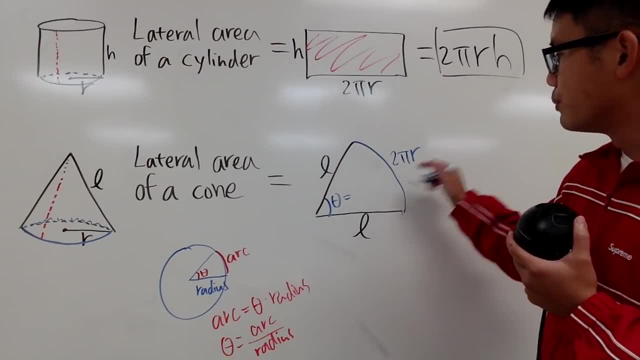 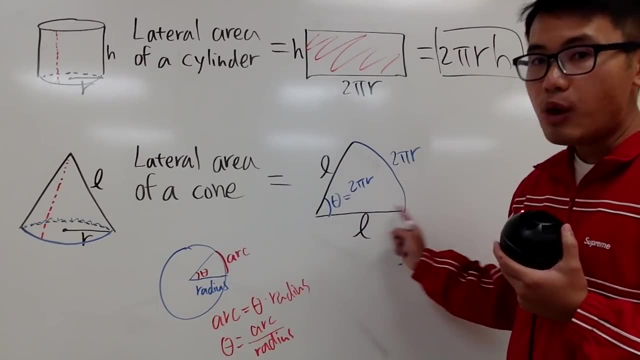 well, I have the arc, which is 2 pi r- Let me just put that down right here- And the radius, you see, is the l right here. So I will just have to divide it by l. So this is the angle that we have. 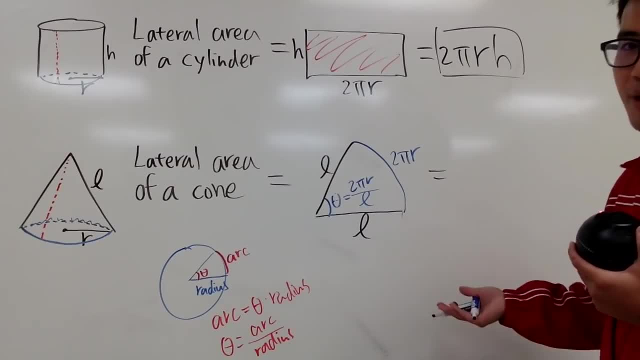 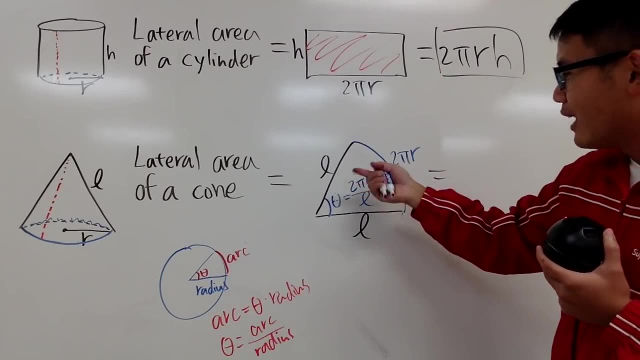 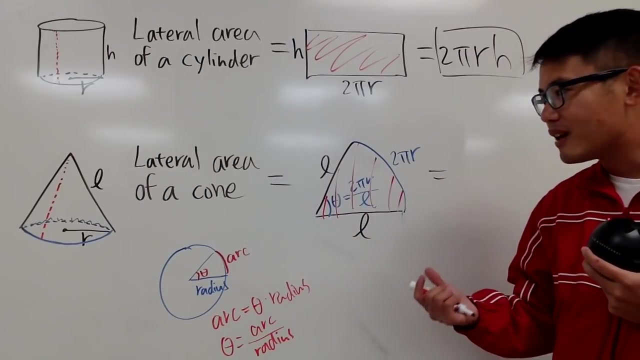 And now to find the area right here. oh, just notice, this is like a box. No, this box is different than that box. Anyway, to find the area of this sector here, recall from my previous video as well, the area of a sector. 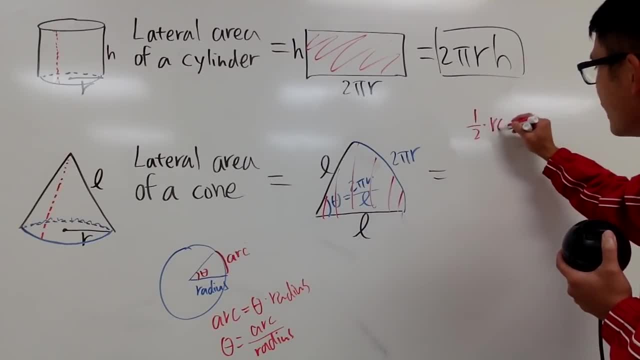 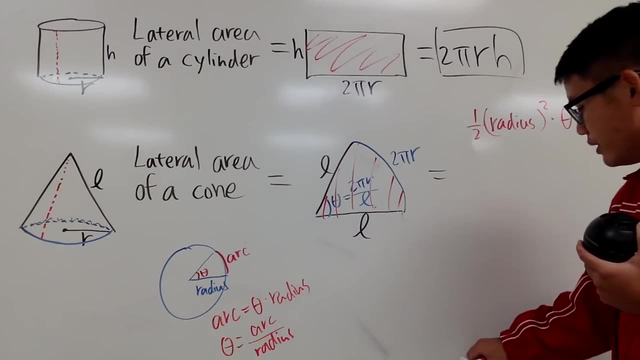 what you do is you need 1 half times the radius and you have to square that times the angle theta. Now let's put everything in action. We need to have what 1 half is 1 half? No brief deal on that. 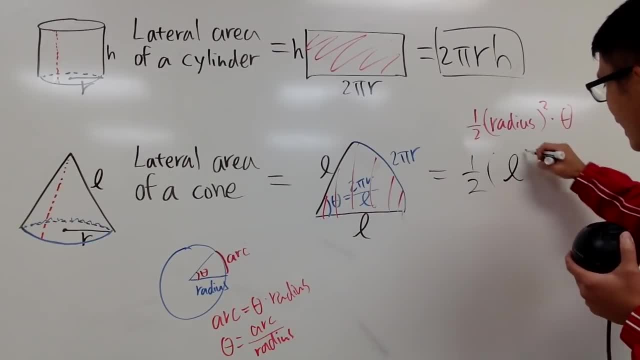 And the radius is, of course, this: l right here, l squared. And then the theta is what? Don't forget, it's this: We have the 2 pi r over l for the angle theta. So this is the angle theta. 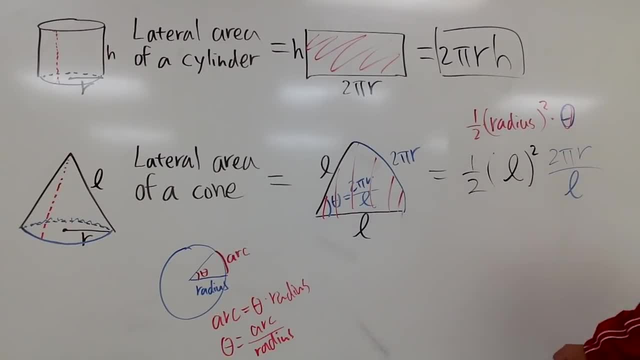 and then we have the radius like that, And once you have this, you can do some cancellations. For example, 2 and 2 cancel and then l to the first and l to the second. here you get l to the first on the top. 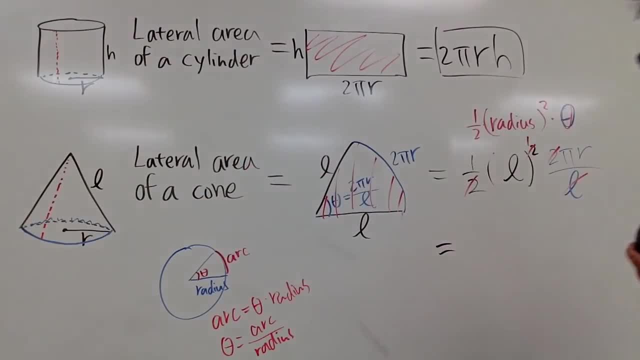 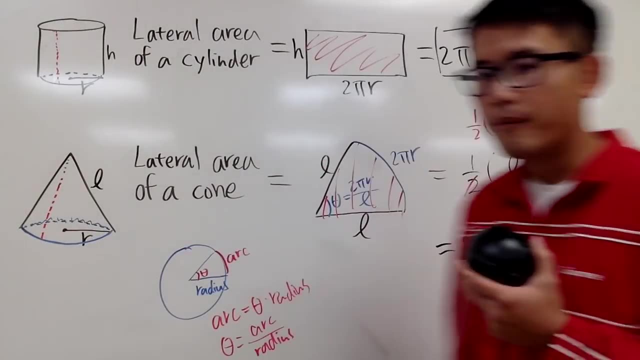 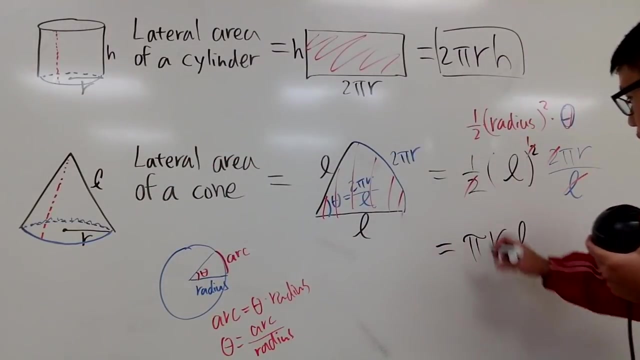 So, all in all, the lateral area of a cone is pi times r, and this is the radius of the base circle. And then you multiply by l, which is the length, the slanted length, like that. So this right here is.